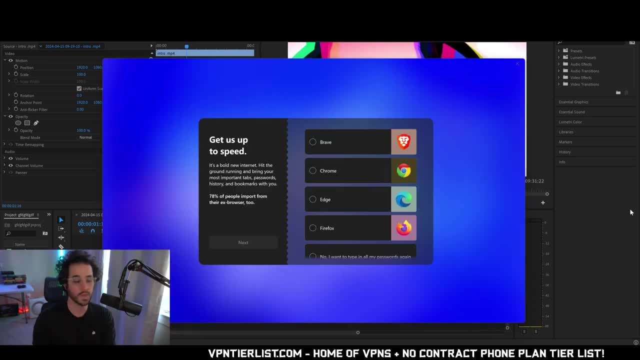 encrypted account. So let's go ahead and do that, All right? so I run ahead and made an account and now we're at the next page. Right here it says: get us up to speed. It's a bold new internet. Hit the. 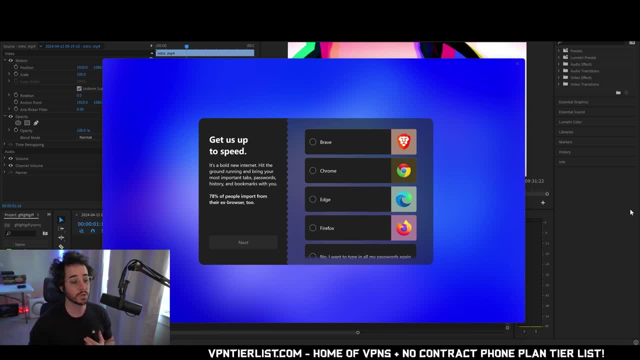 ground running and bring your most important tabs, passwords and bookmarks with you. So that's kind of cool. We get to import stuff into it right away and it kind of guides you through it, which is something I haven't really seen from a browser before. 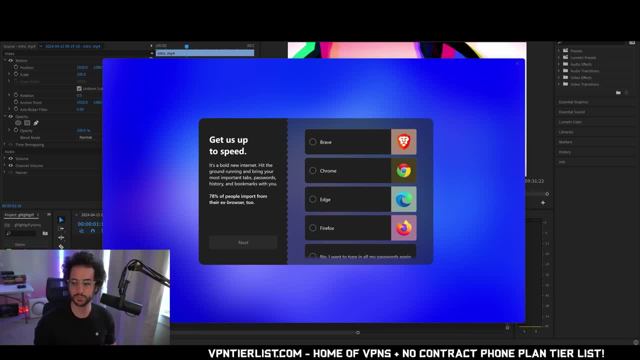 Usually, what this entails is looking up on how to import your bookmarks or something like that. It's kind of standard across the different browsers, but still kind of a nice feature. Next up it's going to say: if you want to make our defaults Right now, I'm going to put no because I'm still 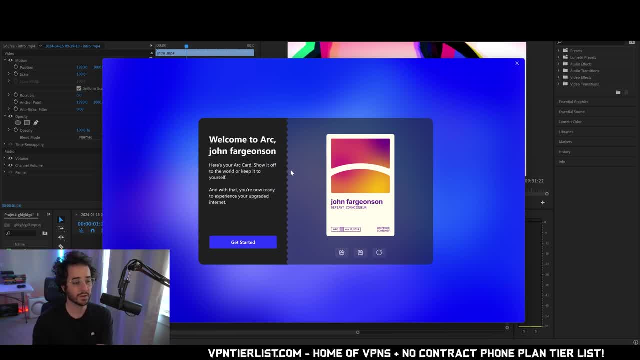 exploring my options. Right here is my ARC card. Show it off to the world to keep to yourself. I guess this is just when I started using it. I made up a fake name, So kind of interesting, I guess. Let's click, get started, Okay, so. 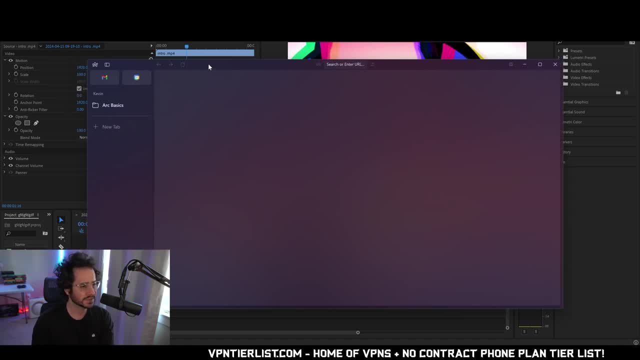 here it is. It's kind of got an interesting color scheme going on, Kind of like a purple Up. here. we have some settings: Check for updates, Standard stuff, New tab. The hotkeys seem to be pretty similar as usual. We have something called spaces, which I'm not sure what it is yet. Tabs, Extensions. 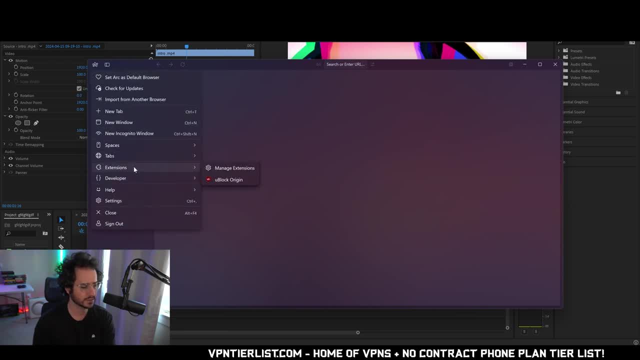 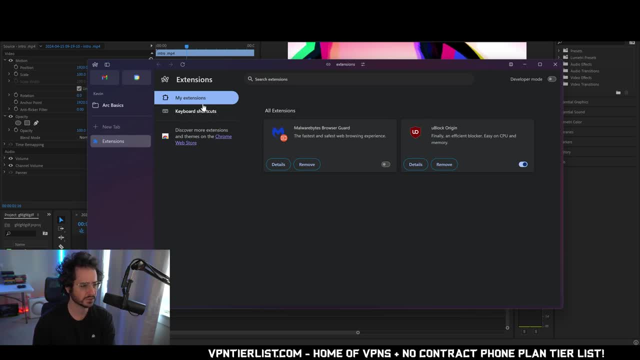 We can go to manage extensions. It looks like it might have kind of imported some of my extensions from my other browser, which is kind of interesting. I'm not sure how it did that, But okay, Well, that makes sense. It's because they're based on Chromium Chrome web browser, So I kind of like 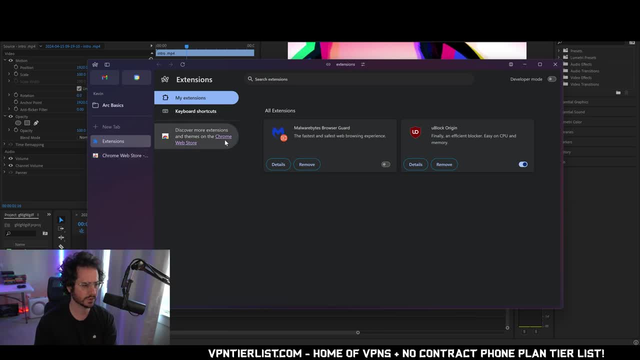 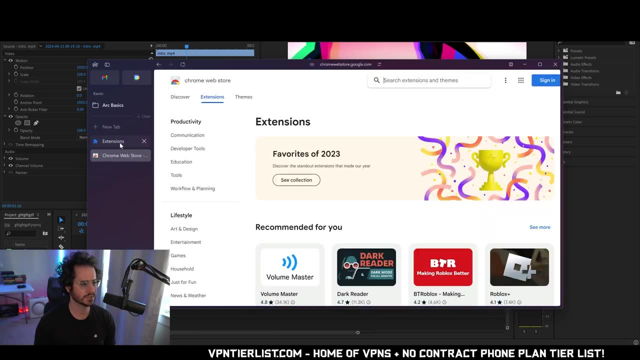 how you could just kind of manage the extensions like this. It's kind of cool. It's a little different than what I've seen integrating this kind of tab here. Well, I guess the reason it is like this is because these are the tabs Interesting, So they're kind of like vertical. 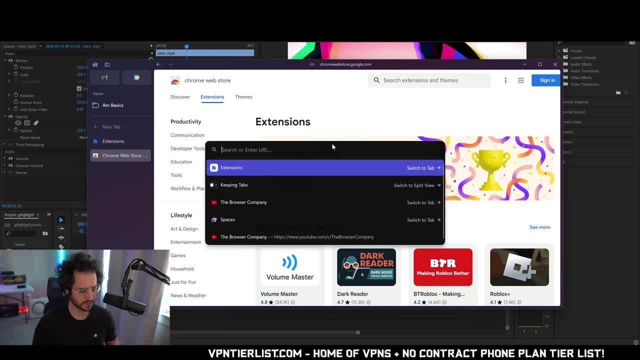 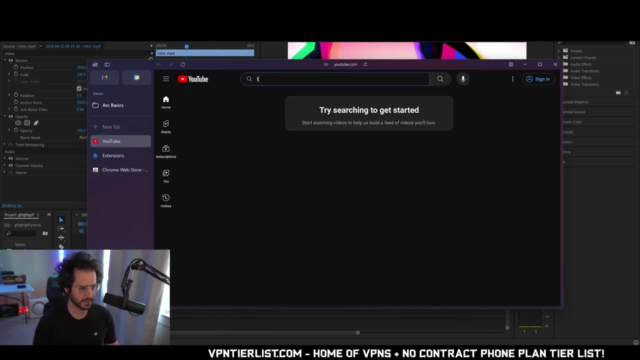 extensions. I've never seen that before either, And of course, if you do that, you will type, And it's like the. the search bar is in the middle of the screen too, which is definitely different. So here we have a basic website pages. We could look at the YouTube channel. Let's see what it. 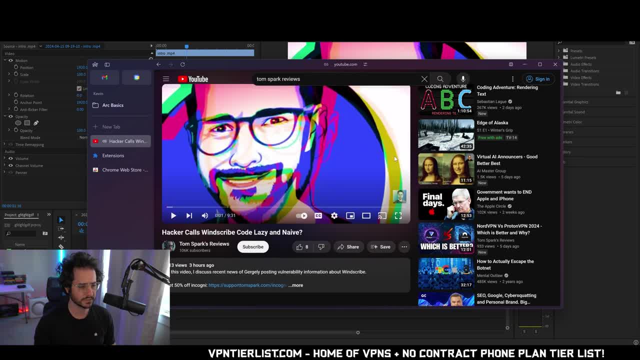 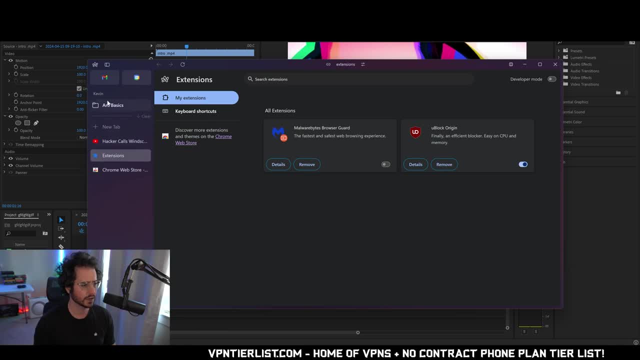 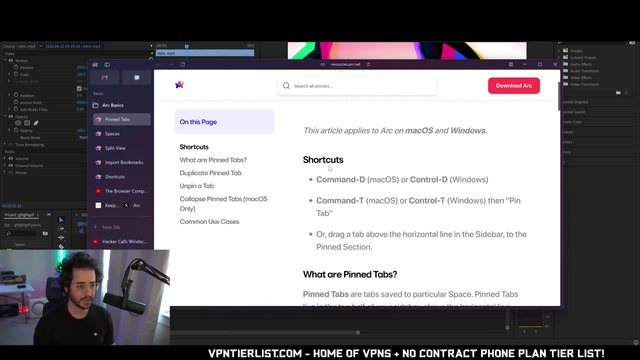 is like you watch a YouTube video. Okay, Seems pretty standard. Nothing too different here, And of course, we have these extensions. So Arc Basics, Here's some kind of pin tabs. So you want to stick around, You could pin a tab. So let's go ahead and try to pin this. 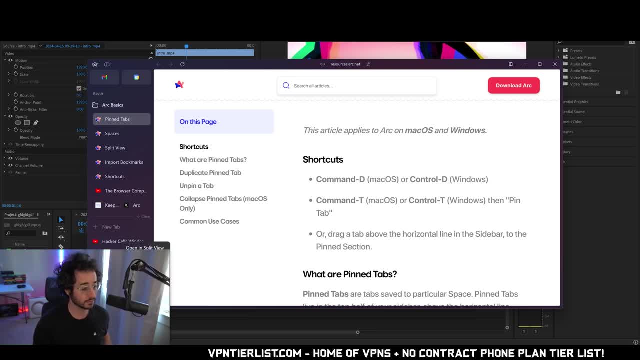 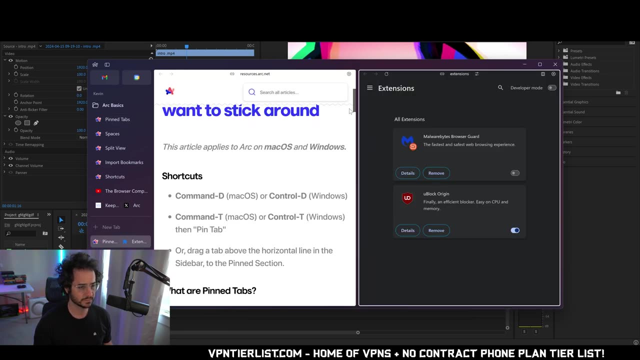 Archive other tabs. Archive tabs below. That's kind of a cool feature. You can move it to pinned. So what does that do? That was pretty cool, So it's kind of like it bookmarked it, Definitely kind of interesting So we could open in split view. Wow, That is actually pretty cool. I could. 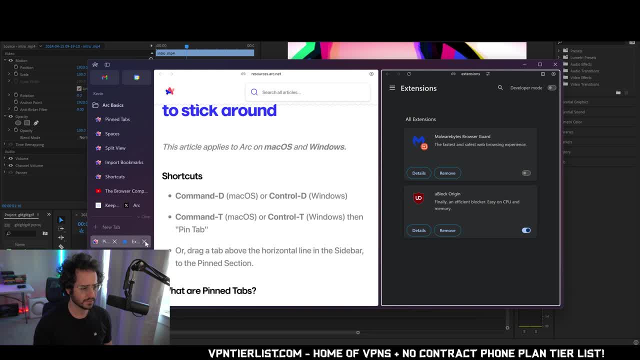 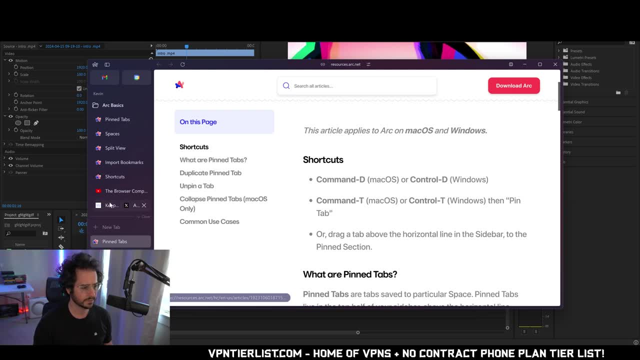 see this being useful for many things. Let's go ahead and see if we get rid of that. There we go Very easy, Nice. So we have different shortcuts. These are talking about pin tabs, So I do kind of like how they integrated the 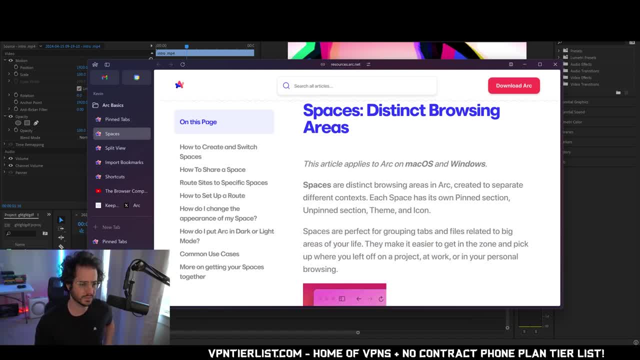 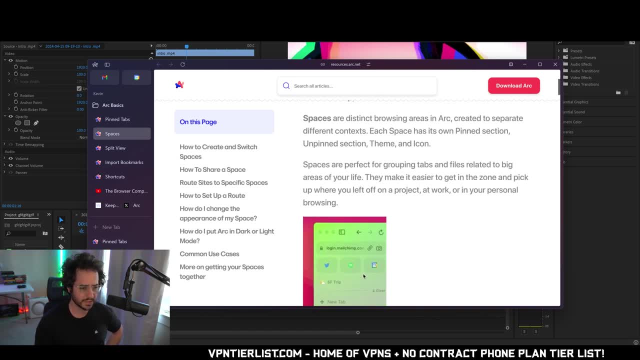 tutorials this way. Spaces. Okay, So this explains what spaces is. Distinct browsing areas. This article applies to archive windows. Spaces are distinct browsing areas created to create different context. Spaces are perfect for grouping files and tabs related to big areas of. 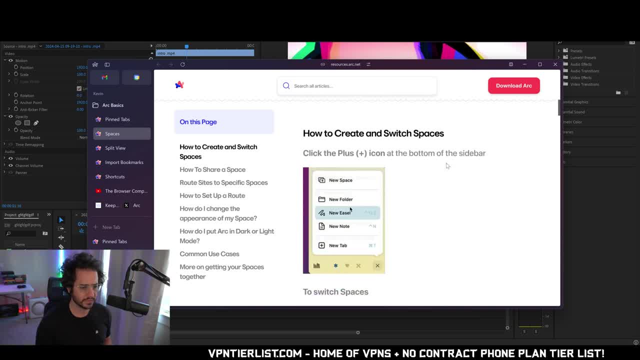 life. This seems like this could be pretty useful. So how do I do this exactly? Click the plus icon at the top of the sidebar. So is it down here, New space? It seems like it's at the bottom. Why does it say at the top? I guess if you want to do it like this you can. Oh, at the bottom At. 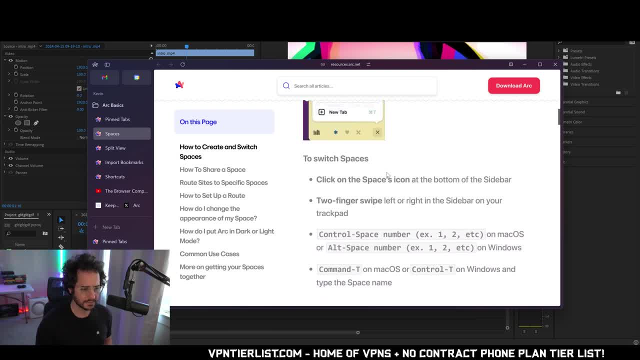 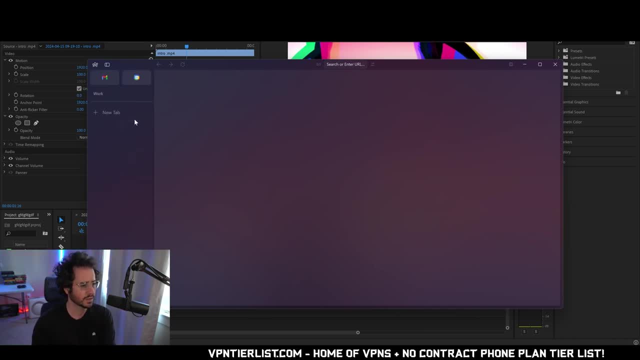 the bottom. I don't know why I thought I said top, So you create a space, So let's go ahead and try that out Space. Um, let's call this work Okay Interesting. So it's kind of like a separate tab interface almost. 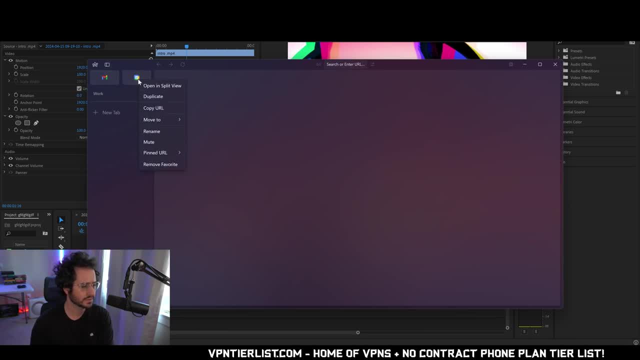 Um, and you could create. what are these things here? This seems to be some kind of like button tab. Um, is this like pin to thing Pin URL? So yeah, it seems to be some kind of pin URL. So how do we go back now? How do we get out of work? Let's see. 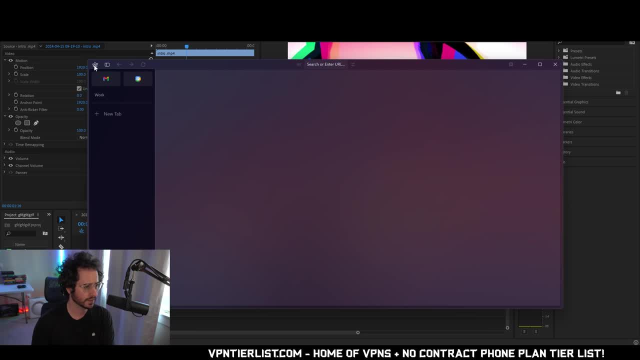 Hmm, How do we get out of work tab? Hmm, Oh, there we go. So it's kind of like a weird little button down here. Um, you can't really see it, cause my thing's in the way. I'll put it over here for now. 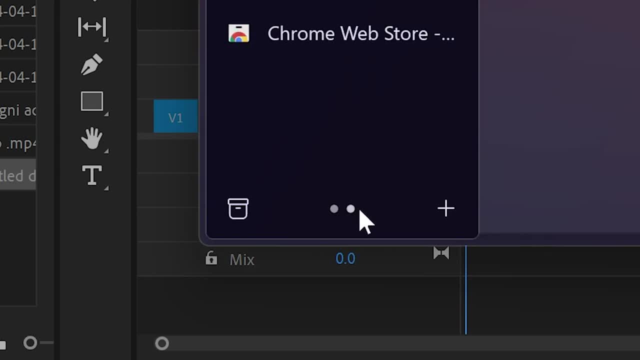 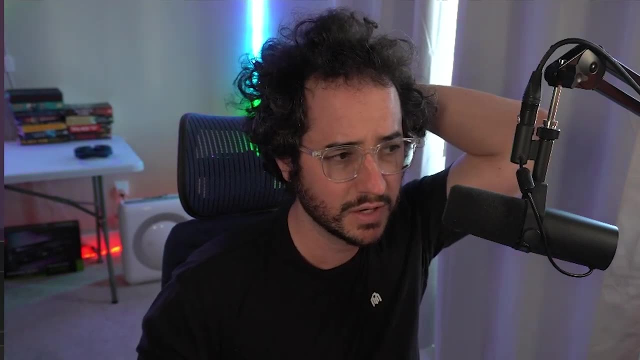 Um, but yeah, it's like a weird little button here where you just kind of clicking back and forth, So that is kind of interesting. You can have separate tabs, always open for various things. Um, so you could have like a slack off tab. Let's read a little bit more if there's anything else. 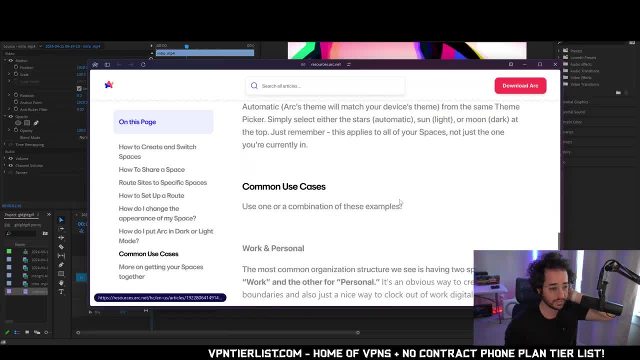 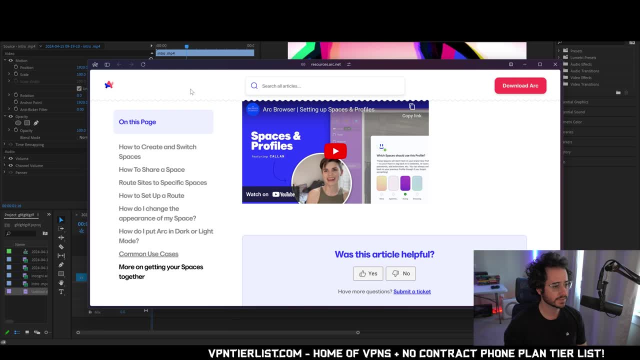 about it. You could also send it to people. Common use case: Work in personal work, in temporary, Cool, All right. So, oh, okay, So you can also kind of get to this like just doing. this is how you bring up the tab menu- Interesting What happens. 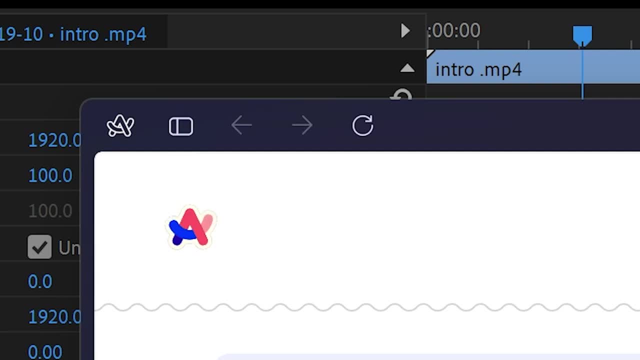 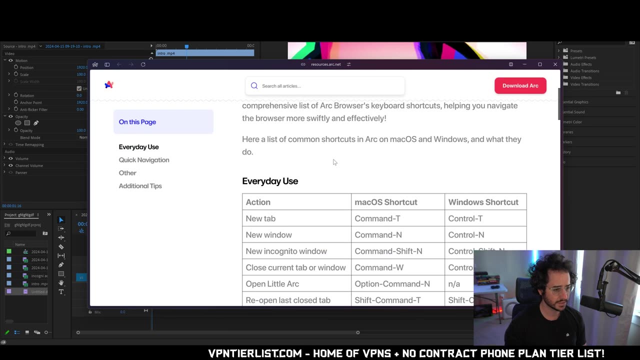 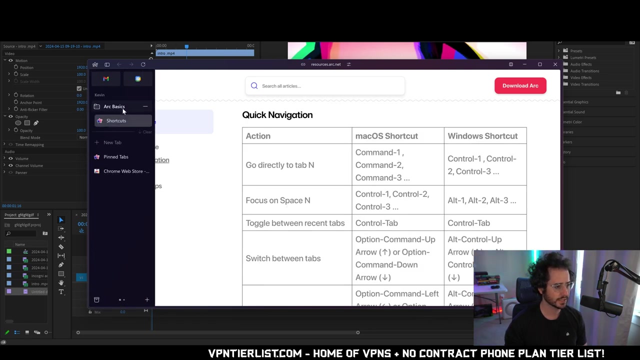 if you type up here: Okay, It just brings that up. Um, you can also share their URL picture in picture. Um, let's go back here: import, bookmarks, shortcuts, anything interesting here Looks pretty standard, All right, So I think we're kind of getting a uh idea of folder. Uh, so you got. 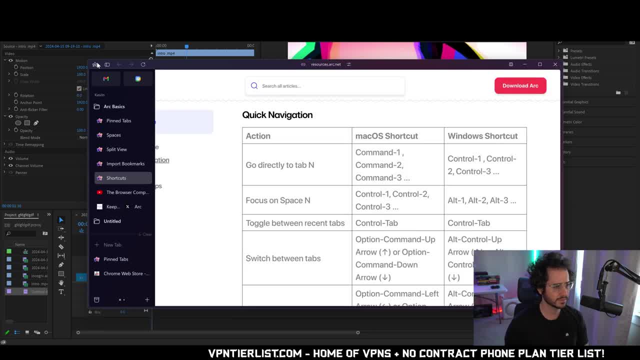 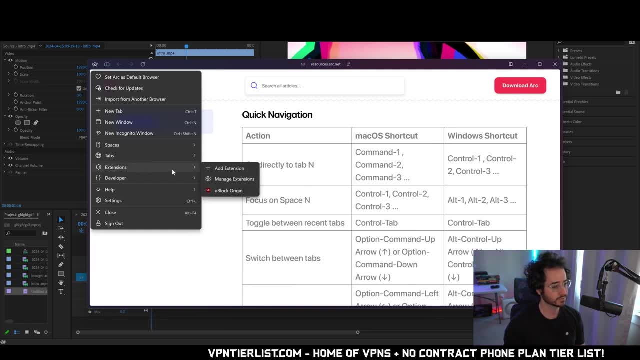 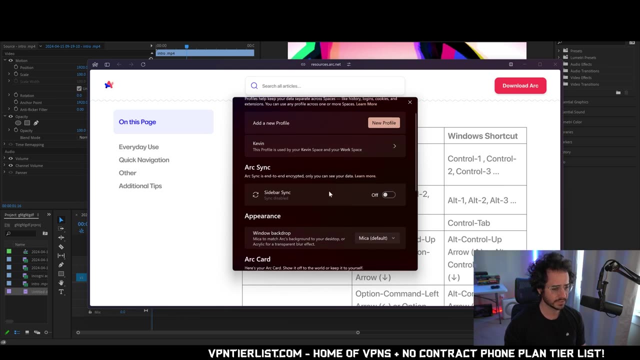 folders. you have different kind of um spaces, which is kind of interesting. There's the spaces tabs um extensions, which is good. Just gonna use Chrome, which is good, Okay, So now we have settings. Let's go look at a settings profile. This is synced to that appearance. Acrylic- What? 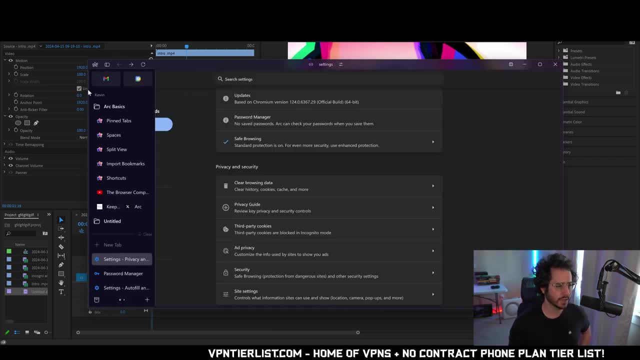 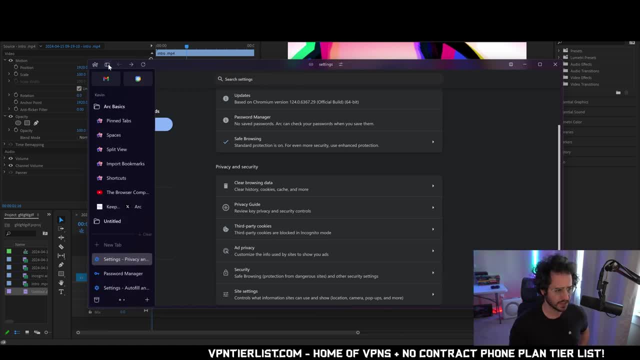 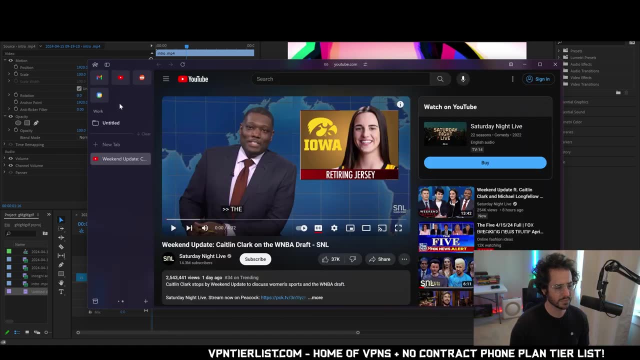 cumbersome um, primarily in these settings. Um, but I do think that there is potential in the split view functionality. That is pretty cool. Um, it is kind of cool how you have little icons, though I I'd say that's like kind of the big difference. Um, so really, you know, at the end 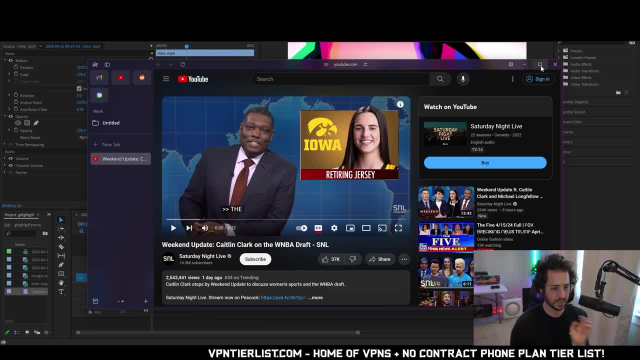 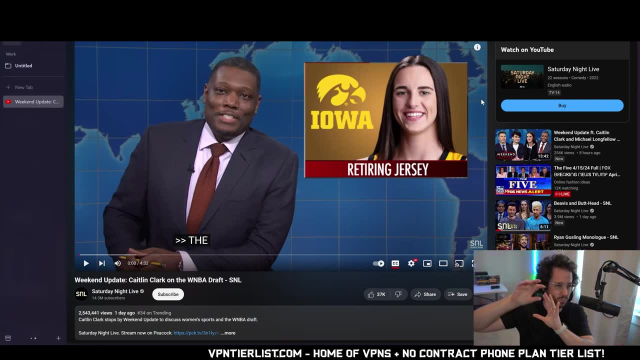 of the day. what is the difference between something like this and something like um Chrome? Well, it's just kind of like they've kind of moved everything from the top to the left and from the top to more like the center, in combination with the. 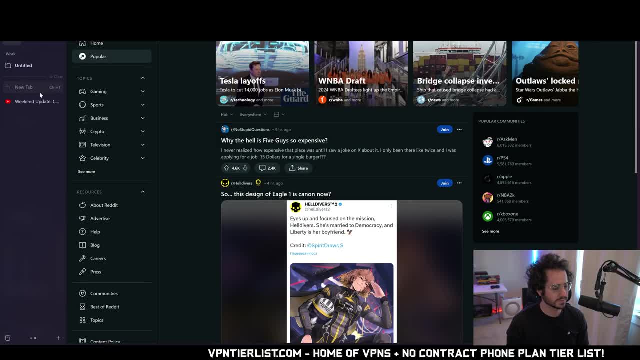 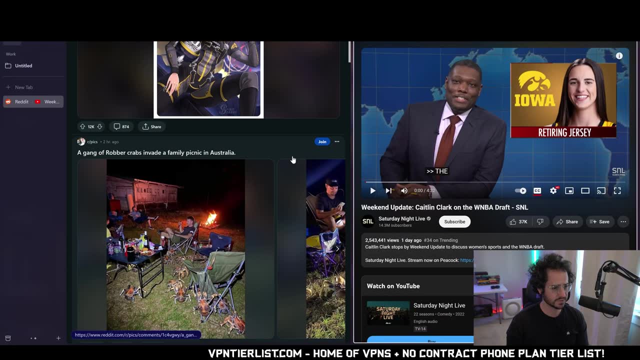 split view kind of functionality. So let's say we open something like this, Um, and then we could do split view, and then we could do something like this: So you can be browsing Reddit while something is on at the same time. So that is like kind of the coolest thing so far that I've. 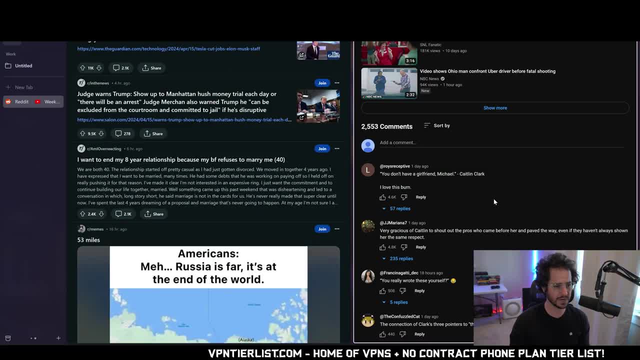 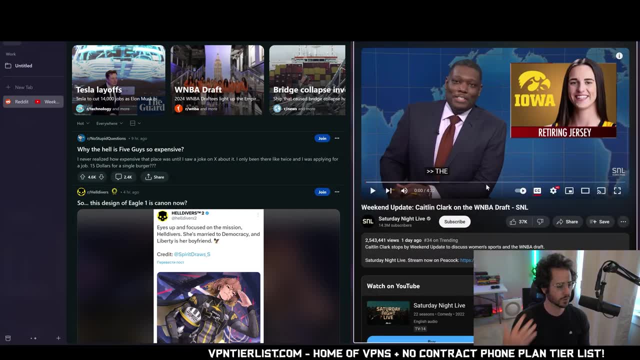 seen here with this browser. I'm not really sure if any other browser can do that, but it does seem kind of like the main kind of thing that it is doing. It works with Chromium extension, It works with Chrome stuff. So, guys, in conclusion, is Arc browser a new internet? Is it? 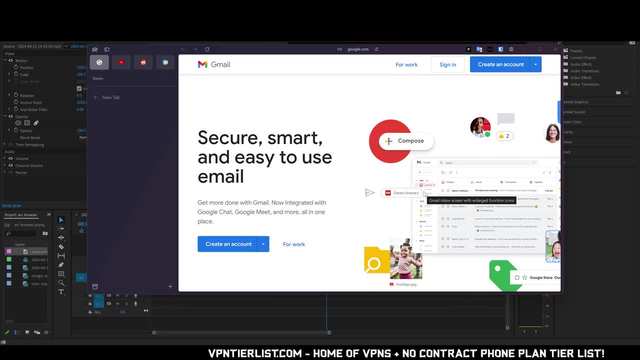 a revolution? Well, I don't really think so. but that said, is it a new replacement to something like Google Chrome that is even more usable? Well, that may, may well be the case. As you can see here, you can see your extensions at the screen very easily. They're easily built in and work. 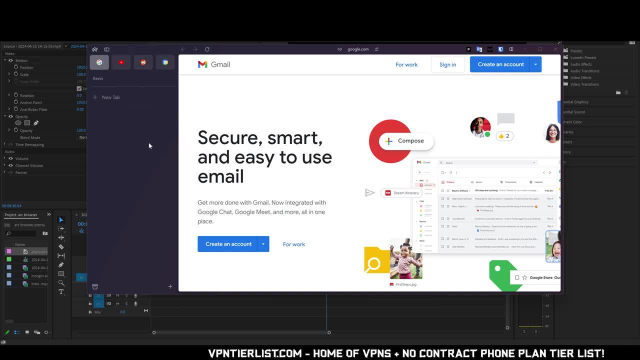 very quickly. One thing I've noticed is I couldn't really figure out how to import my bookmarks, So that could be a point of contention migrating over, or maybe I just didn't figure out how to use it right. Either way it's not working or it's kind of confusing on how to implement them. 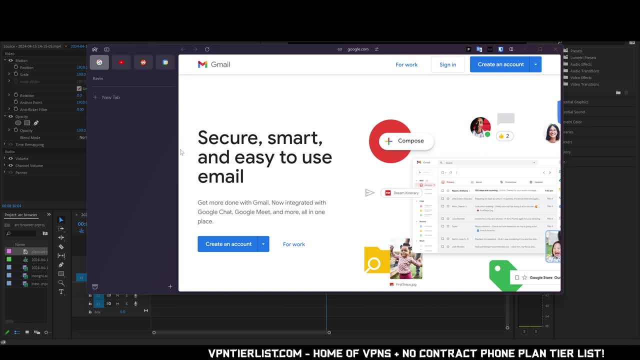 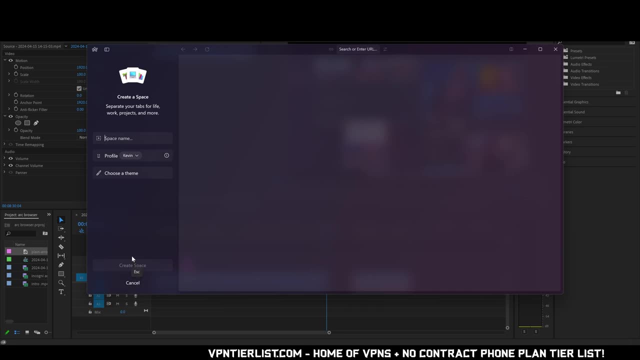 That said, I do think Arc browser's organization of spaces, split, view tabs and things like that is actually better than the traditional way of doing bookmarks. Take, for example, the spaces feature. You can make different spaces for different bookmarks, Different use cases, which is really cool, So you can have kind of different kind of browsers almost. 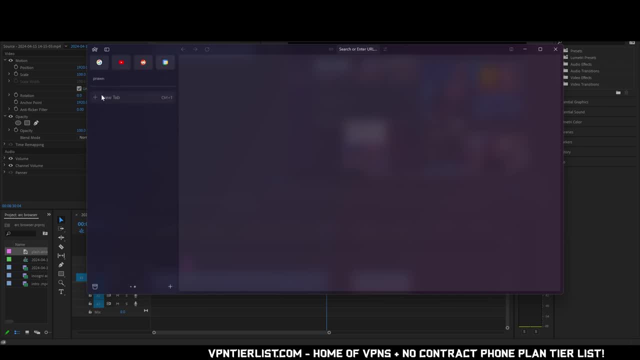 like you want to do, a prawn space. You can have all your different prawn websites that are your favorite one. You can have a work tab or any kind of tab you want for gaming, So you could very easily kind of switch between these different kind of things. It's kind of like having a browser. 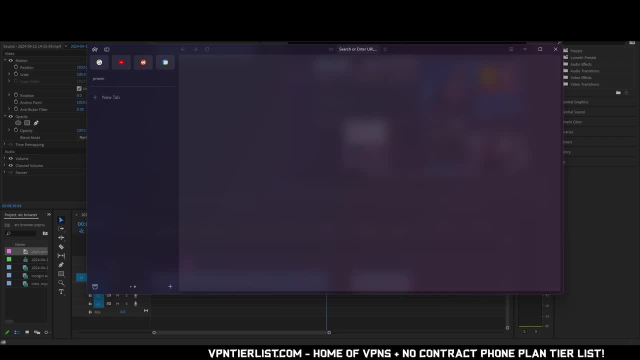 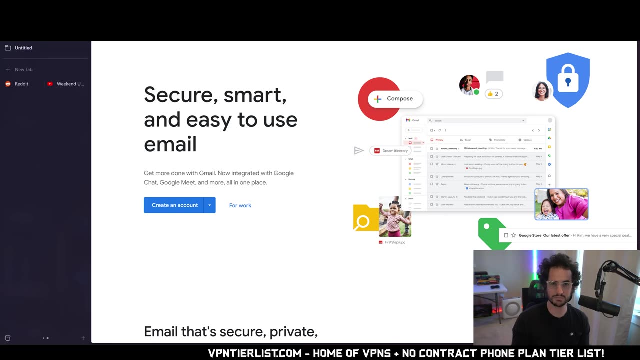 built in a browser at least for different tabs to be available. So it's pretty cool. Definitely can be very useful for organization. So mainly kind of the main thing is like this might seem better at managing tabs is essentially what it does- Managing tabs.